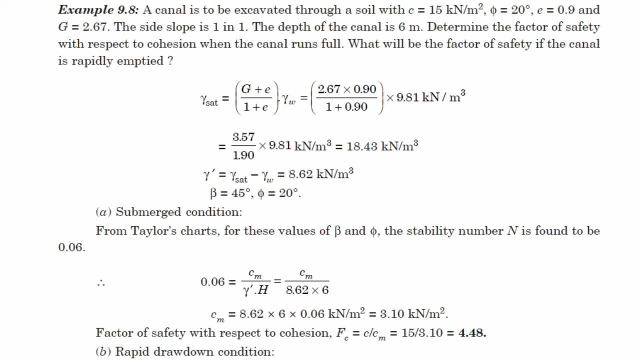 Hello friends, welcome to civil engineering exam. Today we are going to see the problem related with soil mechanics in the topic of stability of earth slopes. So the question is yes, canal is excavated through the soil. with c equal to 15 kN per meter square, then phi equal to that is angle of internal friction 20 degree and the initial void ratio, that is e equal to 0.9 and specific gravity g equal to 2.67.. The side slope is 1 in 1.. The depth of the canal is 6 meters. 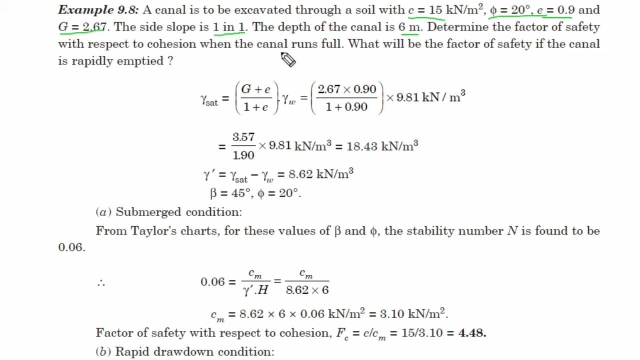 Determine the factor of safety with respect to the coefficient when the canal runs full. So then next question: what will be the factor of safety if the canal is rapidly emptied? So there is a two questions. So first we have to find out the factor of safety when canal runs full, and after that we have to find out the factor of safety if the canal rapidly emptied. So first we have to find out the gamma saturation value. So gamma is equal to g plus e into s, So s equal to 1 because it is fully saturated. 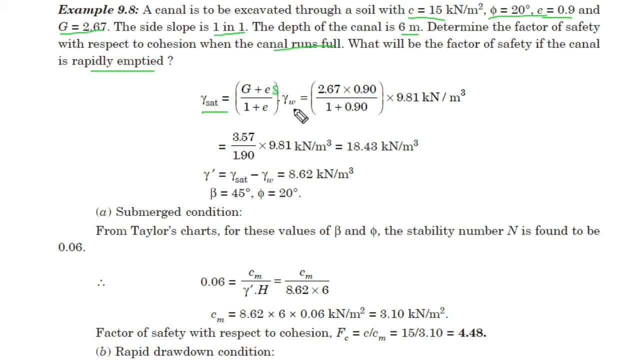 Gamma saturation is equal to g plus e divided by 1 plus e into gamma w. So g is given 2.67 into the void ratio, also given 0.9 divided by 1 plus 0.9.. So solve into 9.81.. So solving this, we got the value of 18.43 kN per meter cube. 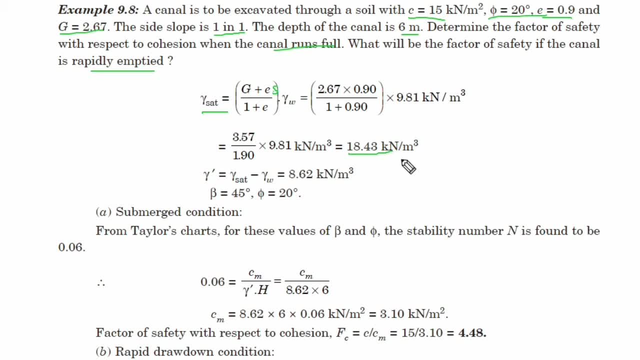 So this is the gamma saturation value. From that we have to find out the gamma submerge. So gamma dash equal to gamma saturation minus gamma w. The formula we know, gamma W is equal to 9.81.. Solving this, we got the value of 8.62 kilo Newton per meter. 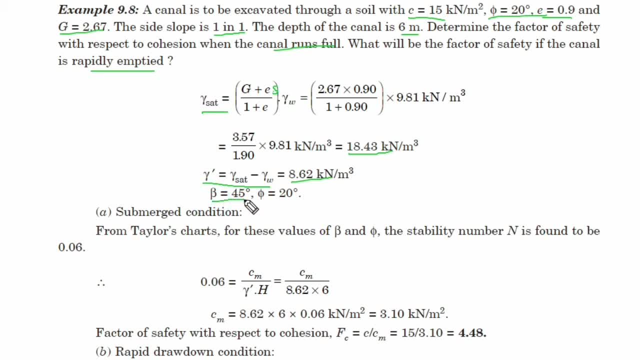 cube. So from that beta is equal to 45 degree and phi is equal to 20 degree. That is also given For the submerged condition from the Taylor's chart. these beta values and phi values, the stability number n value is fine to be 0.06.. From that we know the formula. 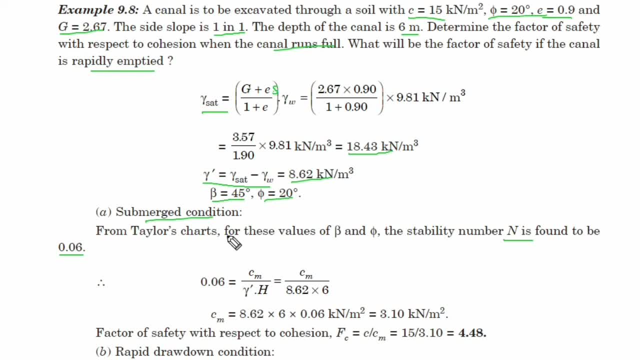 n is equal to Cm divided by gamma dash into h, That is n equal to Taylor's number, Cm is equal to mobilized coefficient and gamma dash equal to that is submerged unit weight and h equal to thickness of the layer. So now we can substitute all the values over. 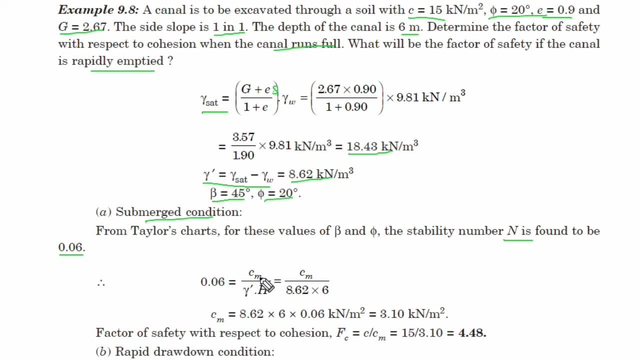 here 0.06 into equal to Cm. divided by gamma dash, equal to the values, we found 8.62.. So we can substitute 8.62 and the thickness is given The 6 meter the canal is. depth is 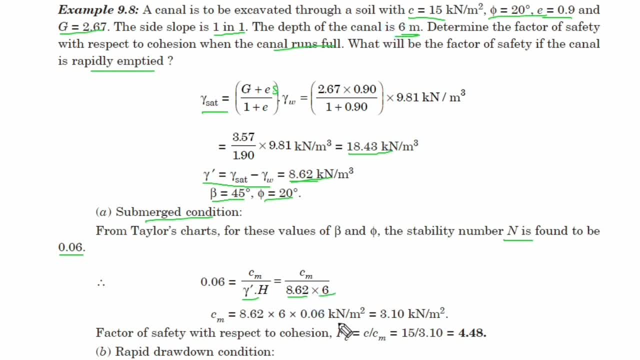 6 meter, So 6, from that we can find out the Cm. So Cm value is 3.10 kilo Newton per meter cube From that factor of safety with respect to coefficient Fc equal to C divided by Cm, that is, coefficient divided by mobilized. 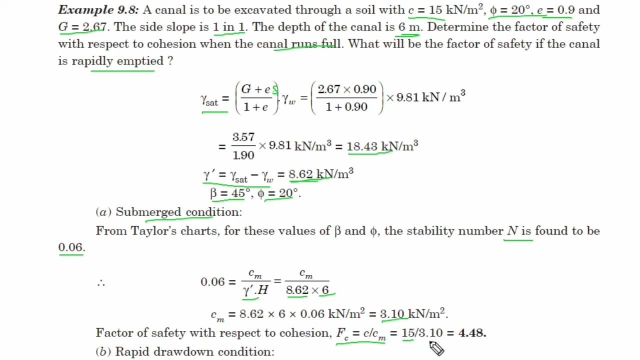 coefficient. So coefficient value is given, 15 is given, divided by, we find out Cm equal to 3.10.. So we substitute over here. So 15 divided by 3.10, we find out the factor. 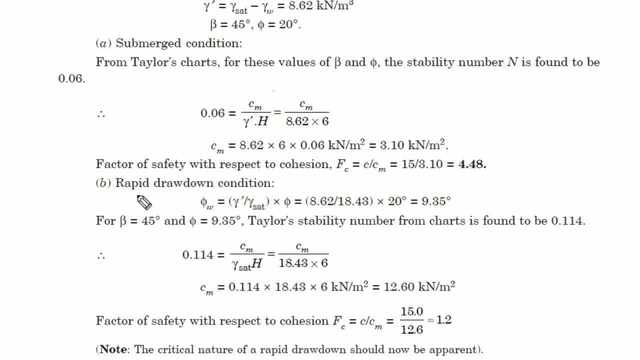 of safety of 4.48.. Now second question, rapid drawdown condition. So phi. phi w is equal to gamma dash divided by gamma saturation into 5.. So gamma dash, we find out 8.62. divided by gamma saturation value 18.43, that is also given into phi value, So phi is equal to. 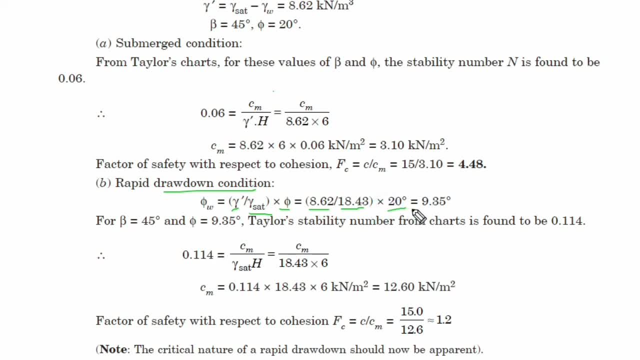 20 degree that is also given. So for solving this, we got the value of 9.35.. For beta is equal to 45 degree and phi equal to 9.35.. So from that, the Taylor chart, we got the value. 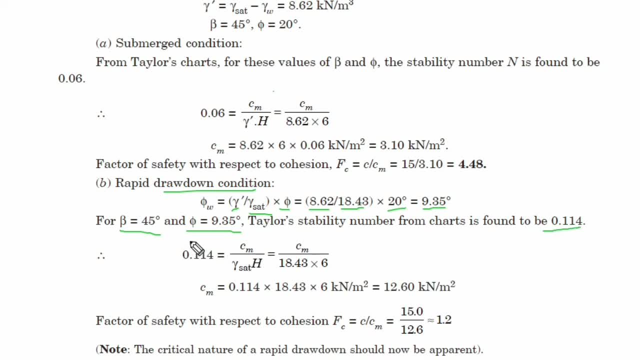 of 0.114.. So now we can substitute all the values. So 0.114 and equal to Cm divided by gamma saturation is 18.43 into h value 6.. So from that we can put submerged condition. we can take in gamma dash value. Here the rapid drawdown: 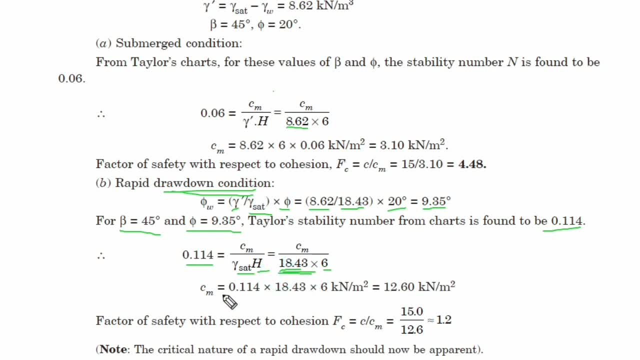 condition. So we can put the gamma saturation value, So now Cm equal to 0.114, into 18.43, into 6 kilo Newton per meter square. So, solving this, we got the value of 12.60 kilo Newton. 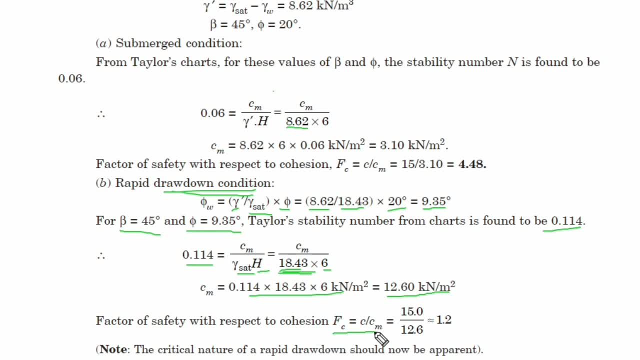 per meter square. So the factor of safety, Fc equal to C divided by Cm, So C equal to 15, and Cm value found out 12.6.. From that we got 1.2.. That is the factor of safety. So this is the method we. 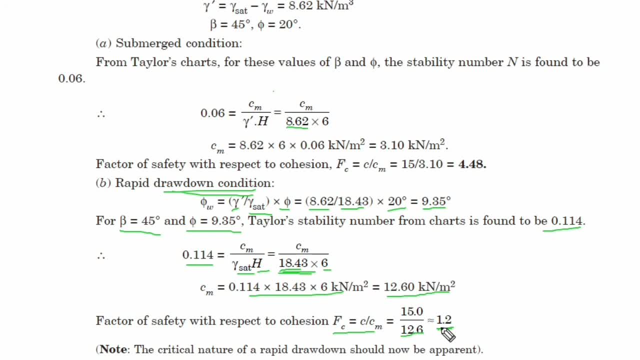 can find out the factor of safety in the stability of slopes. Again, we will see in next video. Thank you. 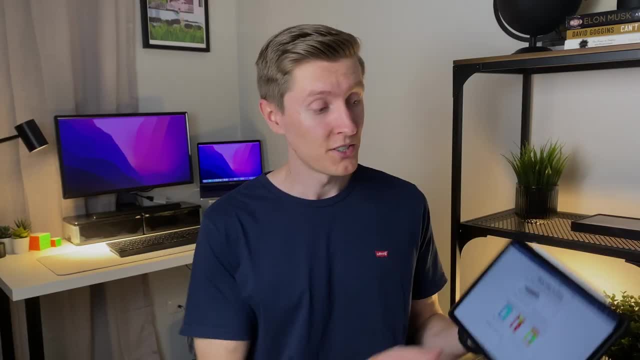 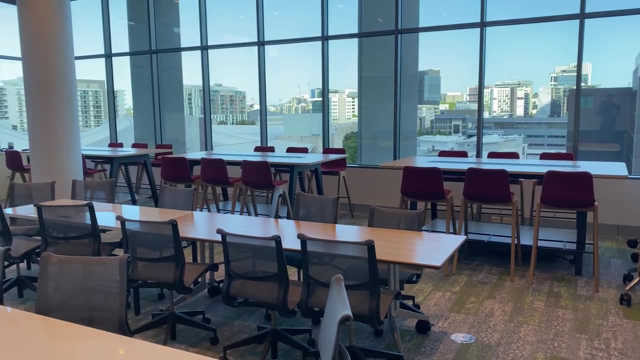 This is a structural engineering portfolio and it's crazy how attaching just two pieces of paper to the back of your resume can become your job landing superpower. As some of you might be aware, I recently quit my graduate structural engineering job at a global design company.